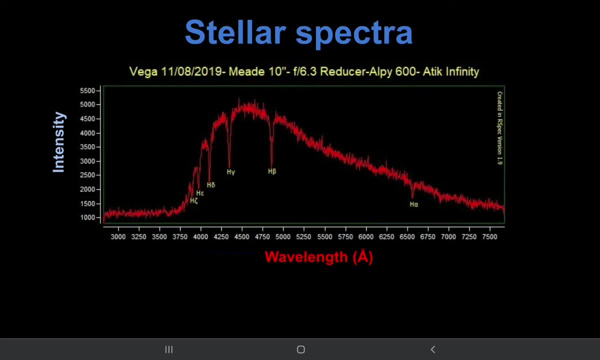 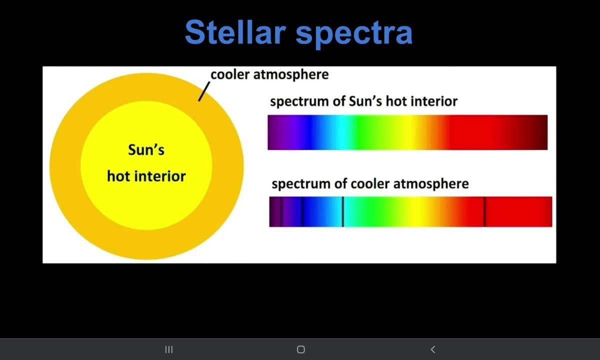 Well, stars actually do emit all of the wavelengths, as you would expect for a black body, And the missing lines are due to absorption spectrum. So from the hot interior of a star you would get a continuous spectrum, as you can see up there on the top right. 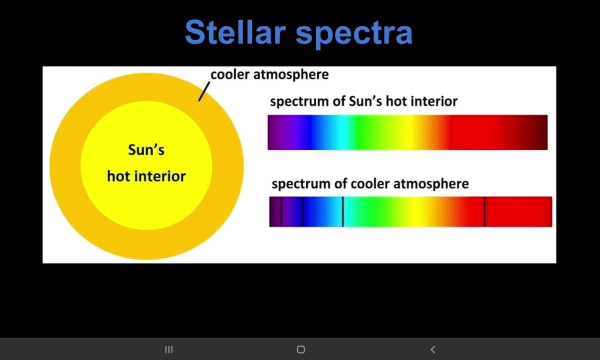 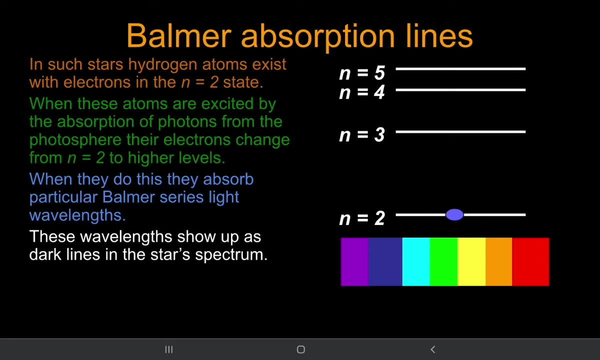 with no wavelengths missing from the spectrum. But what's happening is, as that black body spectrum, as those photons of all the different wavelengths are passing through the cooler outer atmosphere of the star, certain wavelengths get absorbed And to remind you of earlier on in the course, 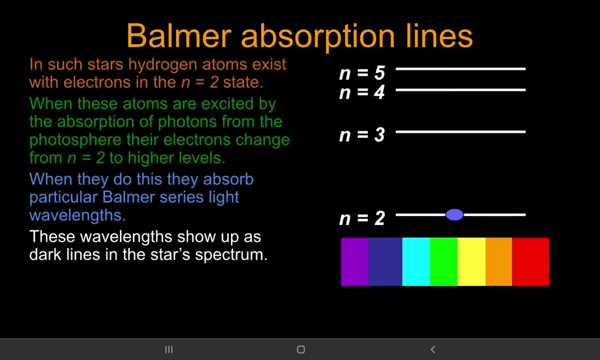 the reason why this happens is absorption by ions, atoms and molecules At A-level. you have to know hydrogen as a particular example. So hydrogen will absorb light in the visible part of the spectrum if the electrons are initially in an n equals two state, so not in the ground state. 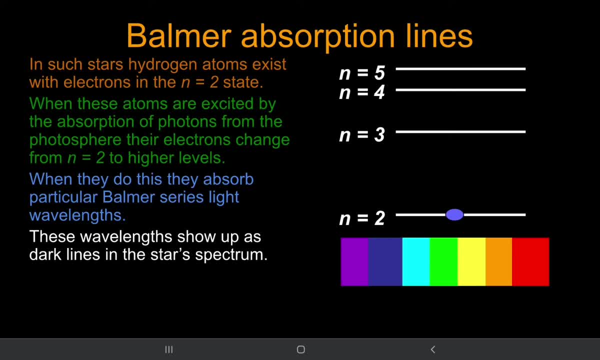 Now, in the very hottest stars, the ground, the electron, will actually be in the n equals two state. So, for example, what can happen is if a red photon is absorbed by the electron, then that photon would have just the right energy for that n equals two electron to move into the n equals three state. 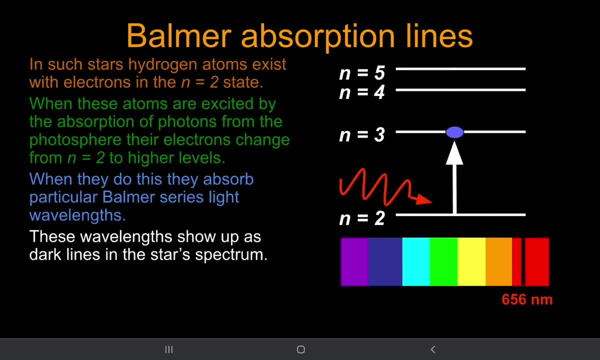 And that means that because that red, that particular wavelength is being absorbed, that there will be a dark line in the spectrum. So there will be a dark line in the spectrum for that wavelength. Similarly, the n equals two state electron could go up to the n equals four state by absorbing a blue photon that has just the right wavelength. 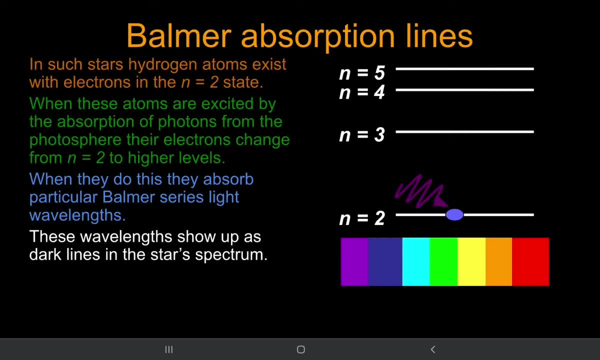 And then there will be a particular spectral line missing. Also, you could have a violet photon, for example, absorbing a photon going all the way up to the n equals five state, And that would mean that there would be an absorption band at that point in the spectrum, in the violet portion. 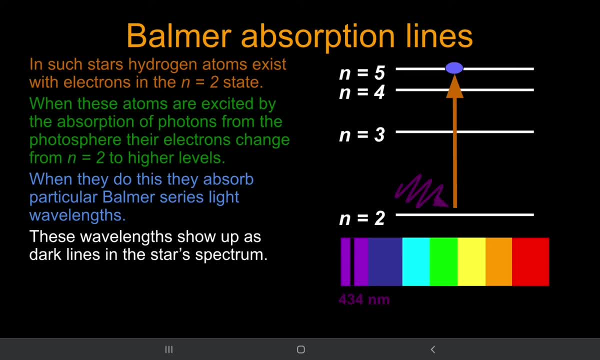 Now, the key thing about these atoms is that they're not going to be absorbed by the electron. The key thing about these absorption lines is that they are characteristic of the species that absorb them. So hydrogen atoms will give very different absorption lines at different parts in the spectra. to helium, for example, 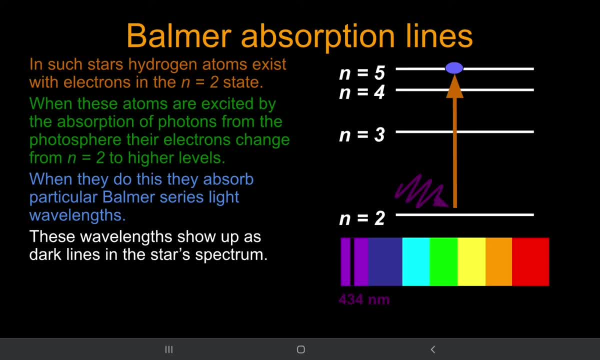 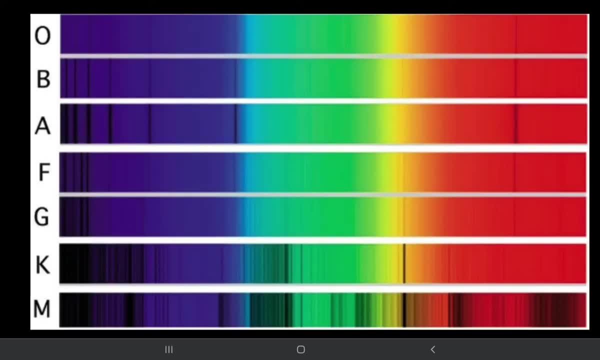 So this acts as a kind of fingerprint for what molecular species are in the outer atmosphere of stars. So what we can do is divide stars up into a number of classes, depending on what spectra you see, And then you can see that there are different types of stars in their emitted light. 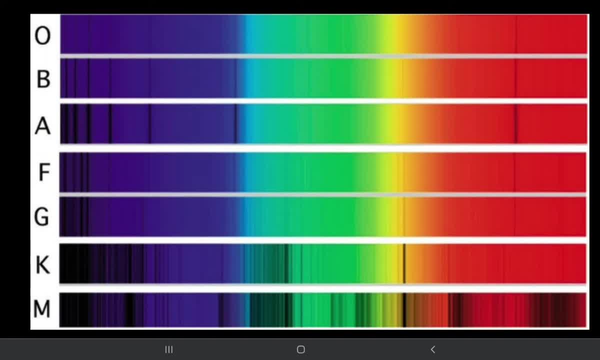 And these seven broad bands are given these letters O, B, A, F, G, K and M. Now we'll talk a bit more about those in a moment. but you can see that the different spectral classifications have very different absorption spectra. 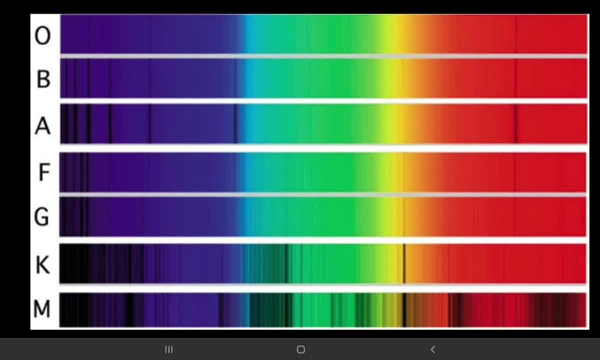 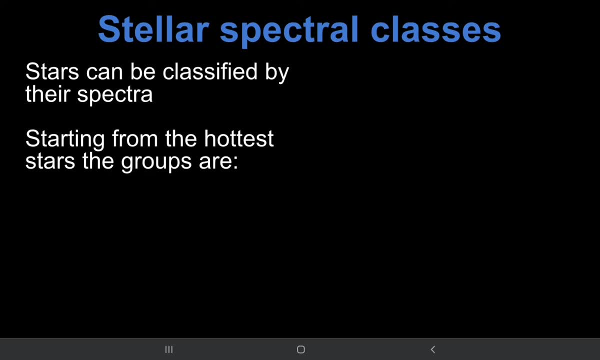 and there are different lines, different intensities in all of them. So these are characteristic fingerprints of different types of stars. Now it was very quickly realized that these spectral classifications also correspond to temperature. So type O stars are the very hottest stars and type M stars are the very coolest stars. 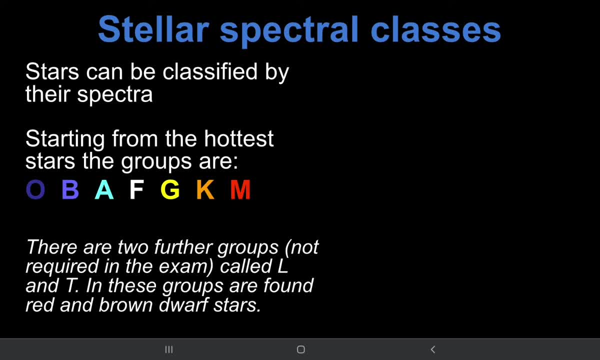 You may see other spectral classifications on the Internet or in books. At A-level you just have to know the seven main ones, And those are subdivided as well into different subdivisions. So for example, you can have an F-class, You can have a 2-star or a B-4-star. 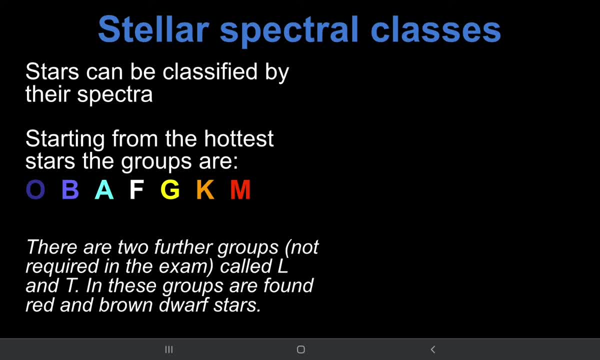 You just have to know the main divisions To help you remember this. there's a little phrase: O B A, F, G, K, M, Or you could say O B A, F, G, K, M, depending on your preference. 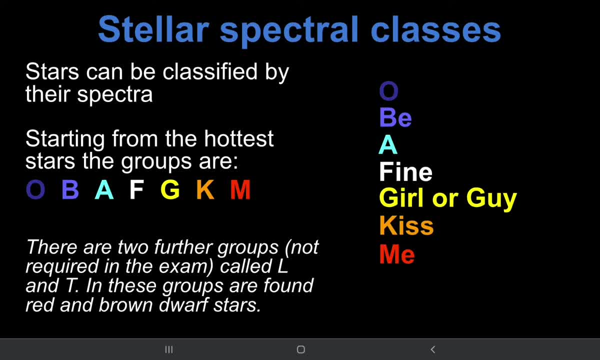 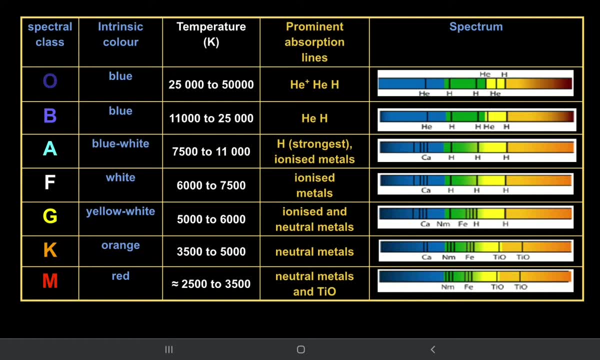 But that little phrase has been used forever and ever whenever anyone's been taught astrophysics. It helps you to remember the order of the letters. So this table of values here kind of summarizes everything that we've been saying, And it's something that you just have to learn at A-level. 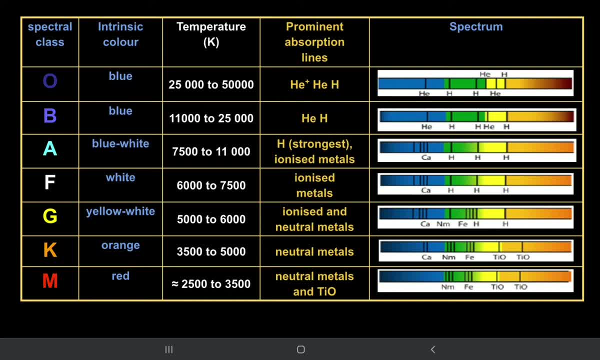 This particular part of the specification is a little bit of a memory test, So you can see as you go down the spectral classes O, B, A, F, G, K, M. you've got blue stars at the top And then as we go down they go from blue to bluish, white to white, to yellow, white to orange and red. 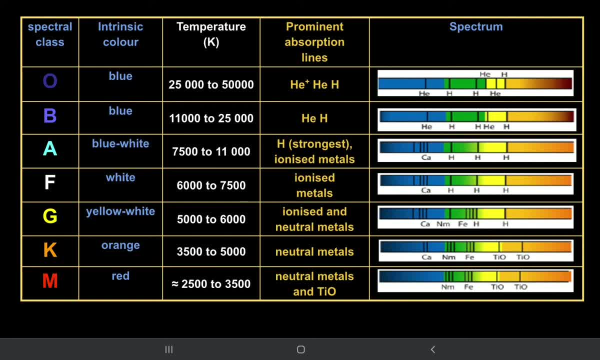 The particular temperatures at which you go from one classification to another classification to another. you have to learn. So, for example, above about 25,000 Kelvin, that's a type O star. You just have to learn those. Imagine. it's just like learning for those of you taking driving lessons. 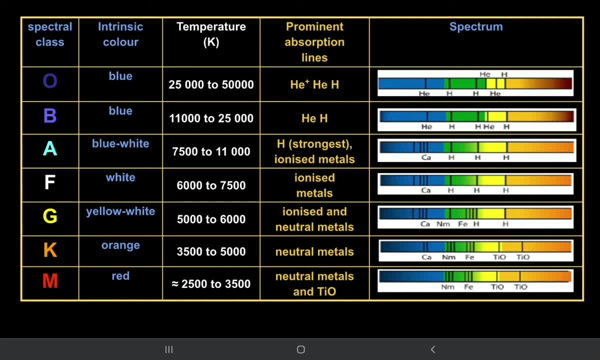 it's just like learning the stopping distances at different speeds, So you just have to learn those temperatures. It goes from about 50,000 Kelvin down to about 2,500 Kelvin And you're going to have to figure some way out to learn those. 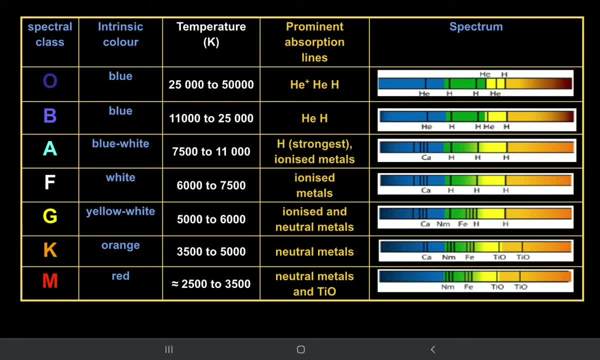 Now there's a correlation with temperature, but there's also a correlation with what species are in the different absorption lines, And so different stars at different temperatures are able to excite or even ionise different species. So let's start at the top. 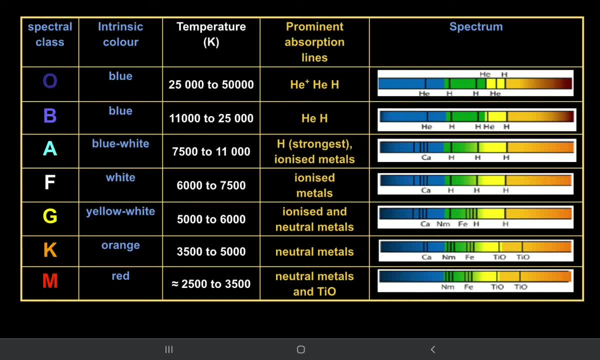 So the very hottest stars have lines due to ionised helium. These are the only stars that are hot enough to ionise helium in significance numbers. now, neutral helium is found in type o and type b stars. it doesn't take as much energy to excite helium atoms into an excited state, so type b stars- you'll also see some absorption. 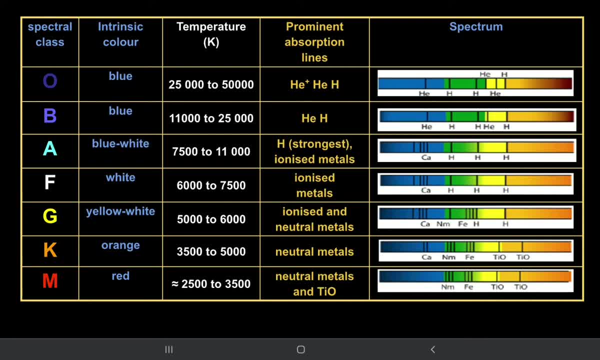 lines due to excited helium, neutral helium. now we've already talked about hydrogen. you will find prominent hydrogen lines in type ob and a stars, and we've already talked about these. electrons must be in the n equals two energy level. in cooler stars, the hydrogen lines are very weak because 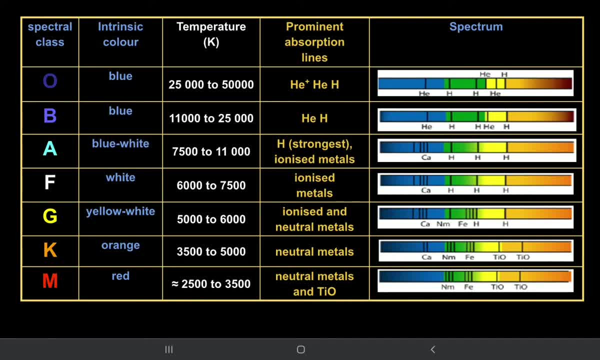 most of the hydrogen is going to be in the n equals one state, so it's going to be in the ground state. the hydrogen lines in the very, very hot stars, the typo stars, are a bit weaker because most of the hydrogen actually gets ionized and ionized hydrogen. 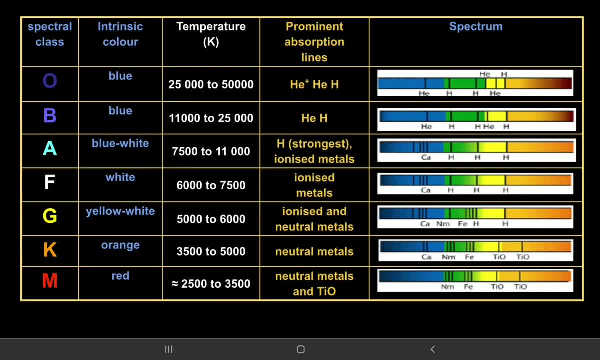 can't produce any absorption lines because it doesn't have any electrons. as you go down the list, as you go from about type a stars down in temperature, you find that you start to see ionized metals. so absorption lines due to ionized metals- now neutral metals- are observed in the 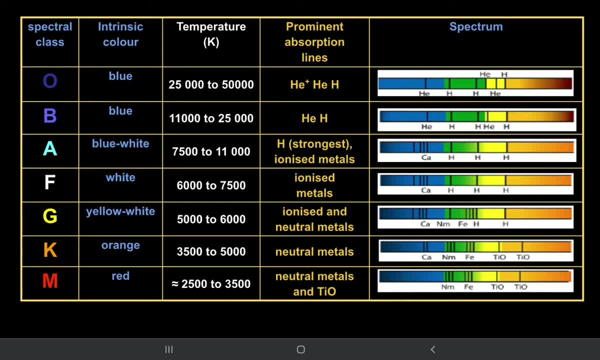 spectra of even cooler stars. these aren't present in the hotter stars. it's not that there isn't, for example, calcium in the hotter stars, it's just that these metallic species would be completely ionized, you know, doubly ionized, triply ionized, so again there just wouldn't be any. 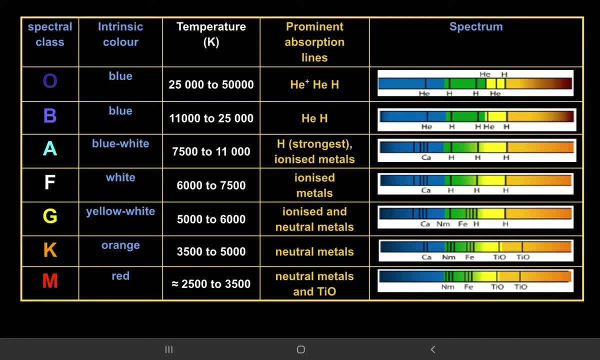 electrons to to hop around and cause absorption spectra. and when you get to the very coolest stars, so maybe k and m type stars, you get absorption bands due to molecules. so the temperature is now cool enough for molecules to exist without them being broken up into the hot stars. so that's a very cool thing to do. so that's a very cool thing to do. 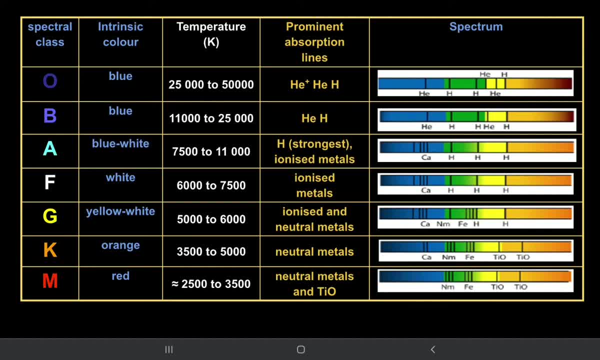 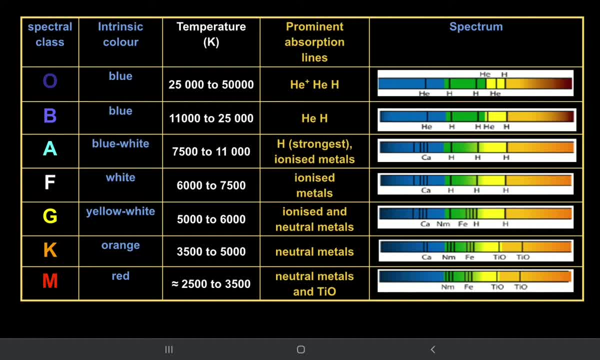 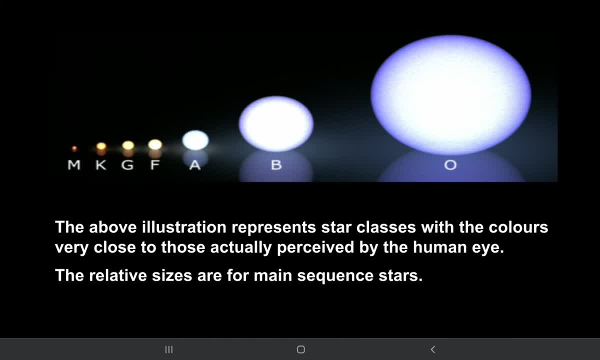 the pictures, you do have to be aware of where they might come from. so if we take our spectral classes, here are the different stars represented with their relative size is accurate. so you can see a few things here. for example, typo stars don't look good. they look kind of blue, but mostly white. the human eye is very good at seeing the middle part of the. 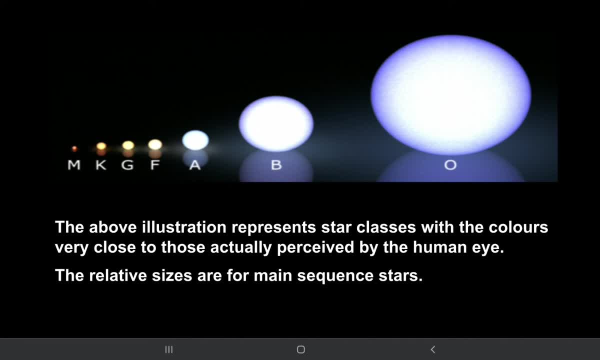 spectrum, the green part of the spectrum, and it's very sensitive to other parts as well, towards the red. so your eye is going to see the blue parts that are prominent, but it's also going to be more sensitive to the green. so you would see that star, as you know. you would almost say it was white, with 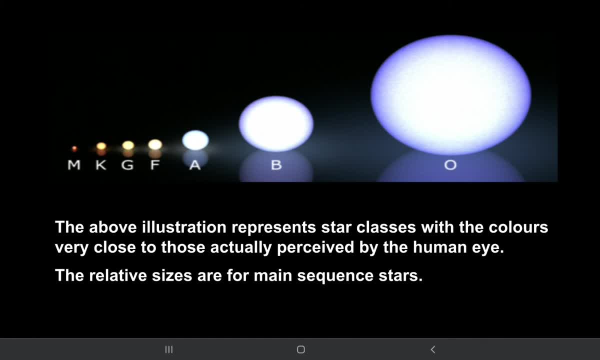 a blue tinge to it. another thing that you'll notice is that the size. as you go from type o star to down in temperature to type m stars, the stars get significantly smaller. now that link between the size of the star and its temperature is no coincidence for a star to get to the hottest. 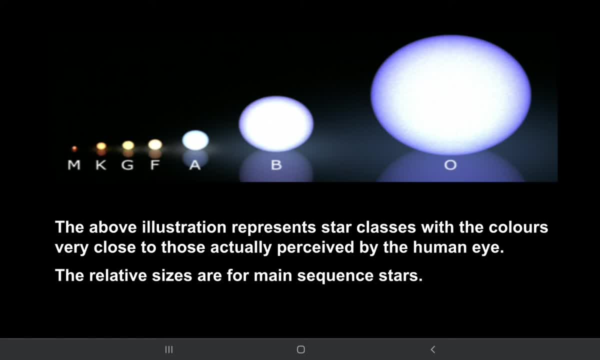 temperatures. it has to have a lot of fusion reactions happening every second. it needs to have a very high pressure and high density interior. and so, because of, because of that requirement, you would, you require lots of mass, lots of mass, lots of gravity for that to occur. we also know from stefan's law that the, the brightness of a star is also linked to its not. 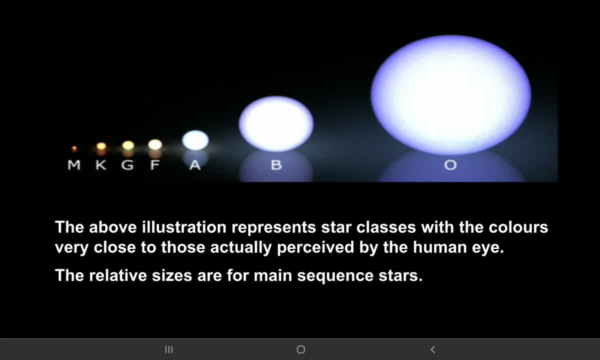 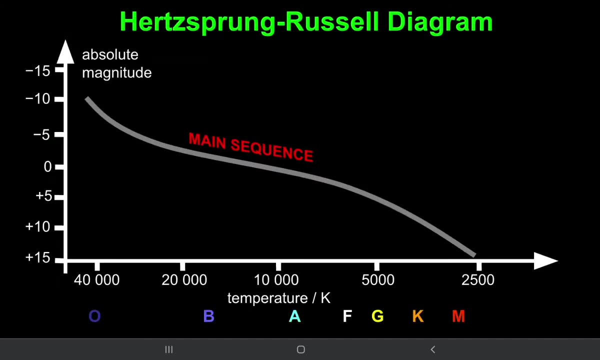 only its temperature but its size, and so you can imagine here that as we go from left to right, the luminosity is going to significantly increase, because not only is the temperature going up, but the size is also going up. a very useful way to see all this information is something called the hertzbrun-russell diagram. 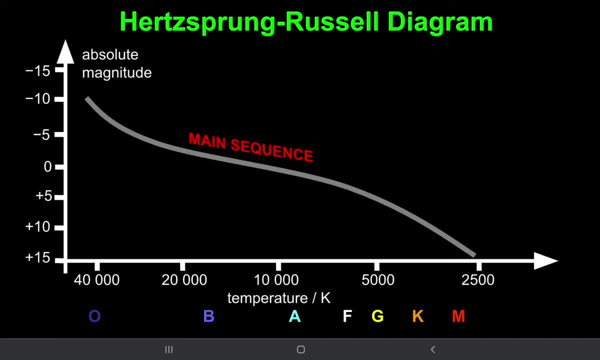 so this is a diagram where on the y-axis you can see the temperature of the star and the absolute magnitude of the star. and you start off with the very dimmest star, so you're at maybe plus 15 in absolute magnitude and you go up in luminosity, so the absolute magnitude is 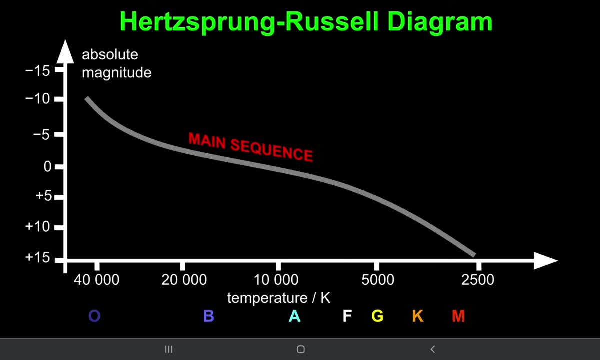 decreasing. you go up, you go down to about minus 15 as an absolute magnitude. sometimes you'll see this plotted as luminosity. on that axis, obviously, luminosity is directly correlated to absolute magnitude. on the x-axis you plot temperature. so you start from about 50,000 Kelvin and you go down. 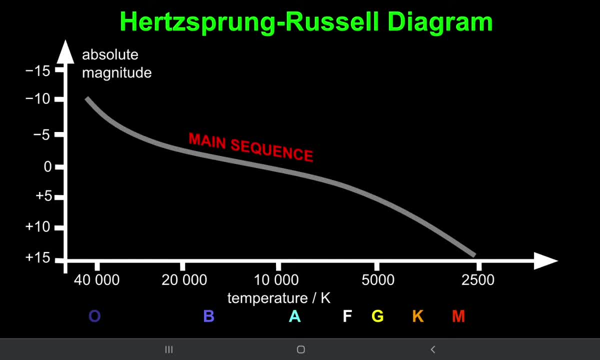 to 2500 Kelvin. the spectral classes are plotted at the bottom with the letters in the middle of the temperature range. so on this diagram you can now plot any star by its luminosity or its absolute magnitude against its temperature. now ninety percent of all stars are on this diagonal band. 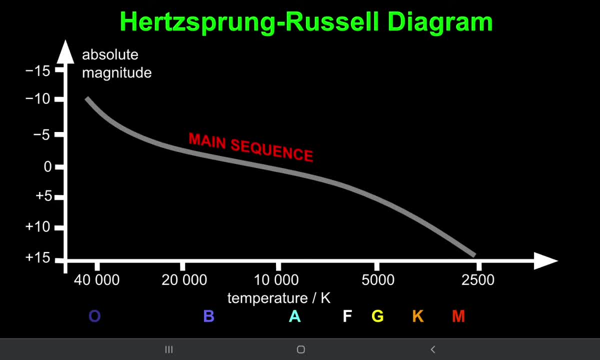 that you can see here, called the main sequence. it goes from the hot, bright stars at the top left down, sloping down diagonally, to the dim, cool stars at the bottom right. so most stars, ninety percent of stars. stars will spend ninety percent of the life on there and ninety percent of stars are in that main sequence. they are very stable. 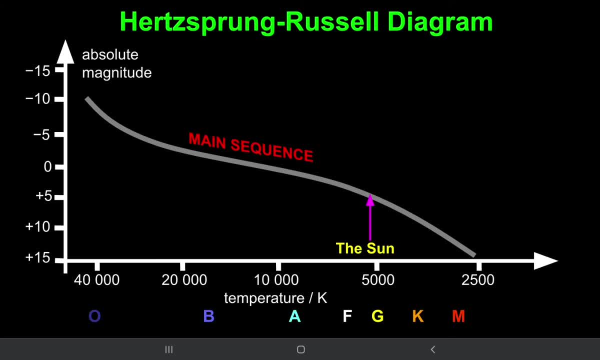 and they last for a long time, as we'll see in future videos. our Sun. you will find it's a type G star, so it's just under 6000 Kelvin. it's actually a G2 star and it lies just towards the bottom corner of the Hertzsprung-Russell diagram. now there are some other. 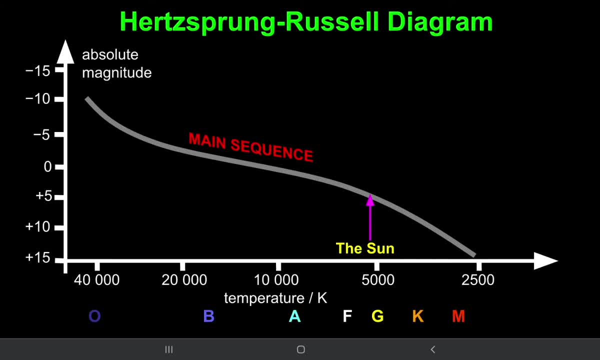 groups of stars that are off the main sequence. so the first group is stars that are low in temperature but very bright, and these are giants and supergiants. the reason that they're so big? well, if you think about Stefan's law, the power, the luminosity of a star is proportional to the size of 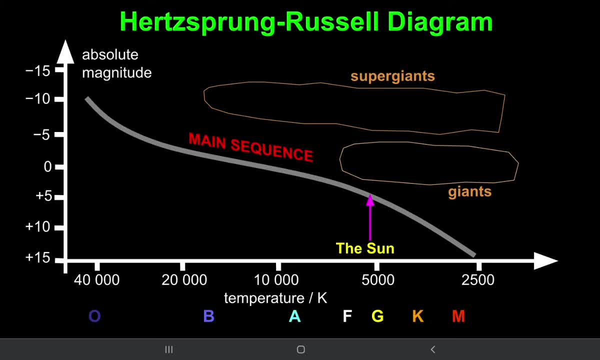 the star on the temperature. so if these stars are very cool but very bright, the only conclusion is that their surface area must be very big, because they're low temperature but they're emitting a lot of light. so those are stars towards the end of their life. another group of stars is in the bottom. 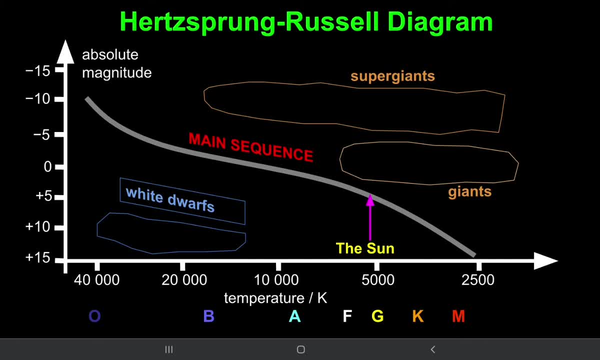 left-hand corner. here these are stars that are very hot but very dim. and again from Stefan's law, if a star is emitting very little light, so it's got a very high absolute magnitude. so if it's not got a very high luminosity but its temperature is very high, the only conclusion: 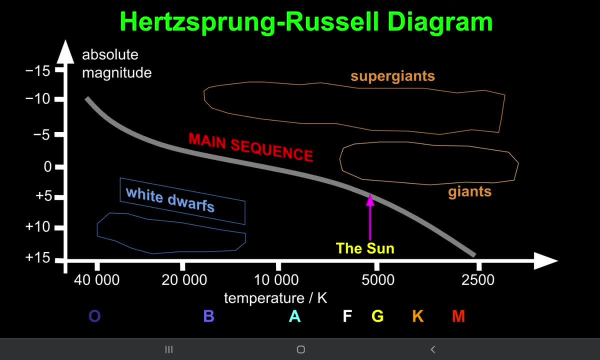 is that it must be very small, that have a very small surface area. so those are the fan in the bottom left hand corner. So what you have to be able to do is, given appropriate data, you have to choose where a star would sit on the Hertzsprung. 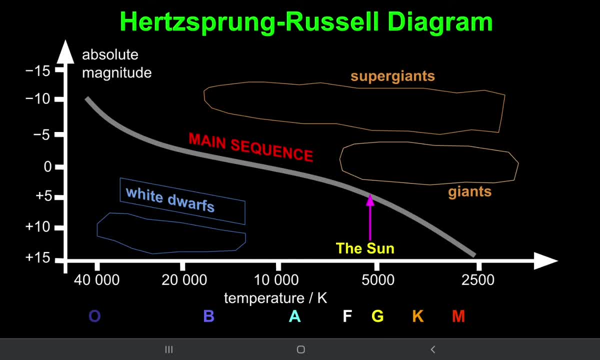 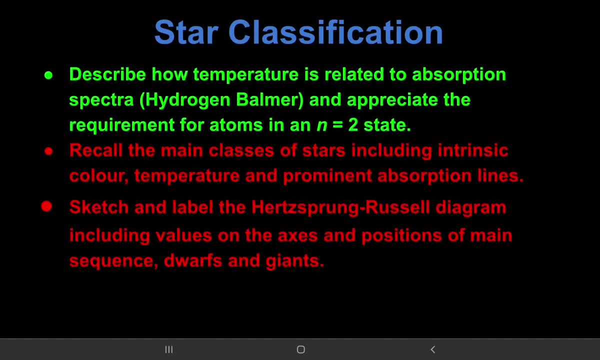 Russell diagram, and in future videos I'll show you how stars move around in the Hertzsprung Russell diagram as they go through their lifespan. So what have we done? These are the things that you have to be able to do. The first is you. 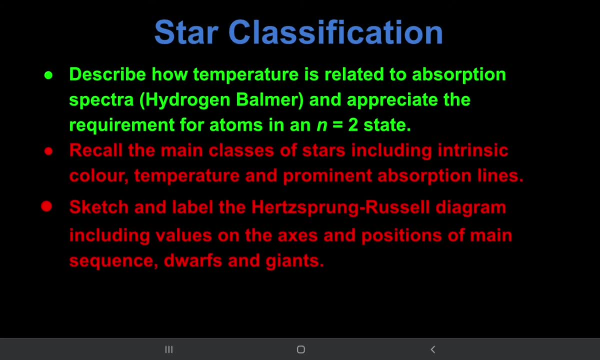 have to understand how the absorption spectra is related to temperature. So, as we said, the very hottest stars even have ionized helium in their spectra and as you go down you start to get hydrogen in the spectra and then you start to get ionized metals, and then metals that are not ionized and even molecules as you go. 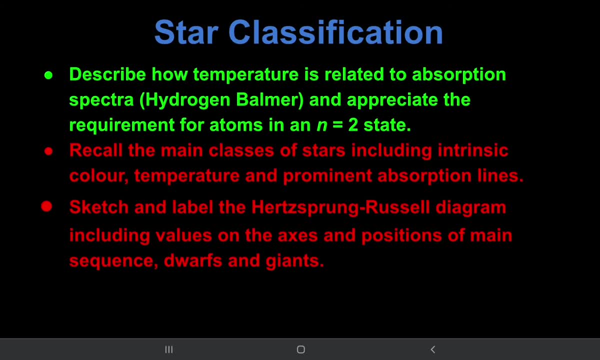 down in temperature. You have to particularly understand why hydrogen in the visible part of the spectrum requires the n equals 2 state. The ground state of hydrogen wouldn't work. You wouldn't get spectral lines at the right wavelengths. The next thing we did. 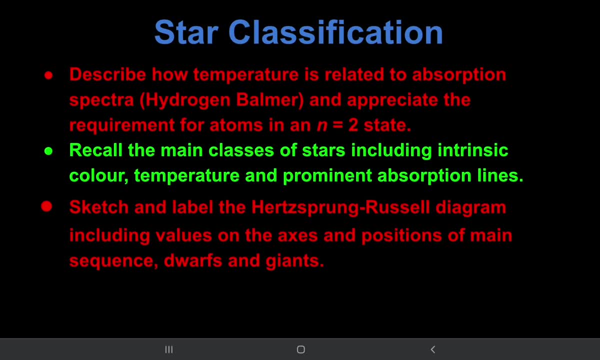 is. we went through the seven spectral classes. You just have to learn them. You have to know their colors, their temperatures and what the prominent absorption lines are, What molecules or ions are giving rise to the absorption lines. Remember the phrase OBFY and go kiss me as a way to remember the letters. Finally,